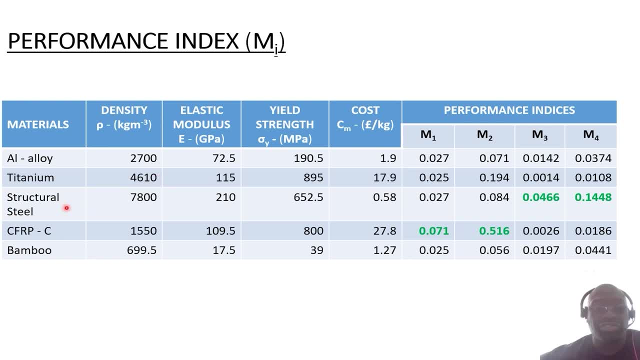 cube, titanium 4610, structural steel 7800, carbon composite 1550 and bamboo 699.5, the elastic modulus. so for aluminium 72, structural steel 210 and bamboo. so again, this is clear to view. however, you can also include a differentiating factor. 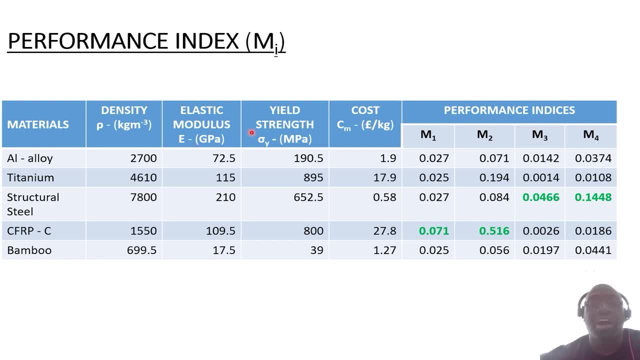 so here we're going to look at what the impacts of these indices are when it comes to cost. so what are the implications? so the first metric, or performance index, m1, looks at the stiffness parameter, so stiffness to density, and when we put these values, so we put in 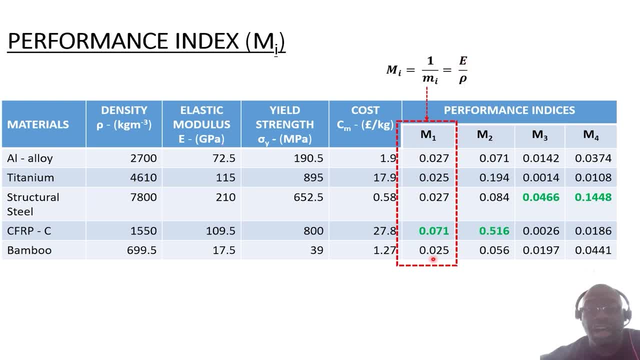 structural set and now we need to look at what is the difference between the density and the different types of mass and the density of the material we get, and we want to have a more precise and common idea of the density of the material, so we use the last metric. 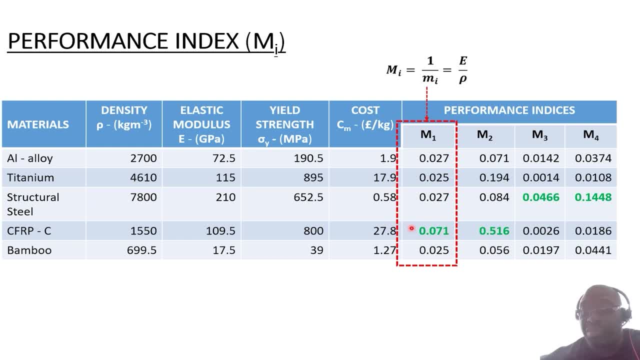 so what we see here is a decrease in density and we find that if we use a more normalLucy, again we can look at metric two. so this time we're looking at the strength to mass performance index, m2. so we'll be using sigma y over rho and again putting the values that. 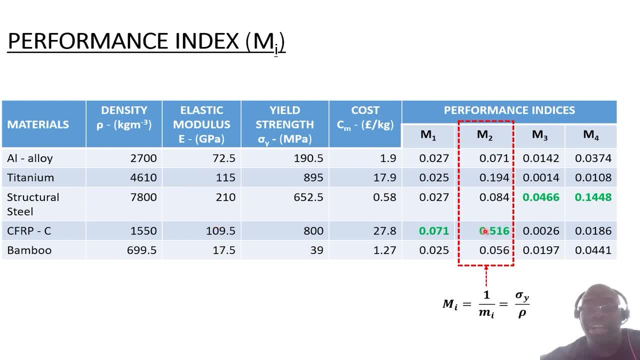 we've extracted from the material database is indicating that carbon fiber is the best material. but what happens when we introduce the cost element? so when we introduce the cost element? so again, what is, you know, the matrix per cost? it then changes things a bit. so, in this regard, 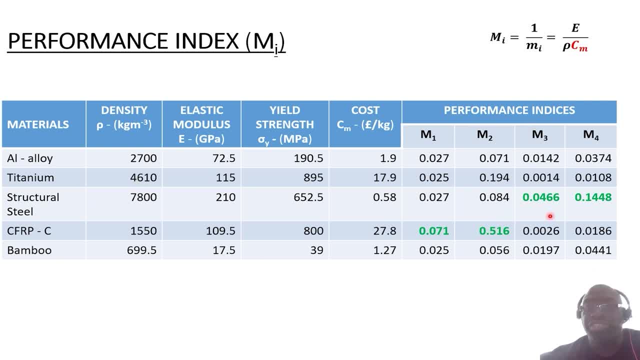 we are. we're now having a structural steel exhibiting the best value for money. when we're looking at stiffness to mass and when we're looking at strength to mass again, it's indicating that structure still be the best material to choose. so it kind of makes sense. 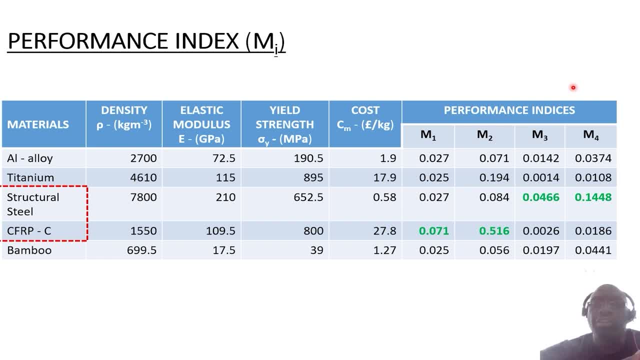 as to why, when it comes to mass volume production of bicycles, structures still tend to be the most common material used in fabricating bicycle frames. however, when it comes to bespoke or low production volume or bicycle frames particularly towards a high-end market and where the performance is important in 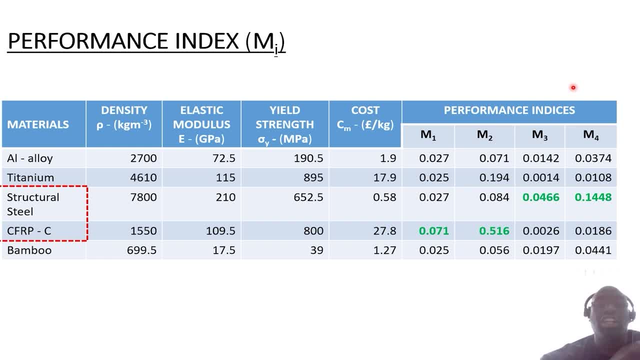 terms of strength, stiffness, to you know the light weightness of a given bicycle design, then carbon fiber is the common one, or the best material to use, as indicated by the performance index. so, again, you can use this approach in conjunction with CES to enable you, you know, filter and identify the best material. you know that your outline objectives governs. 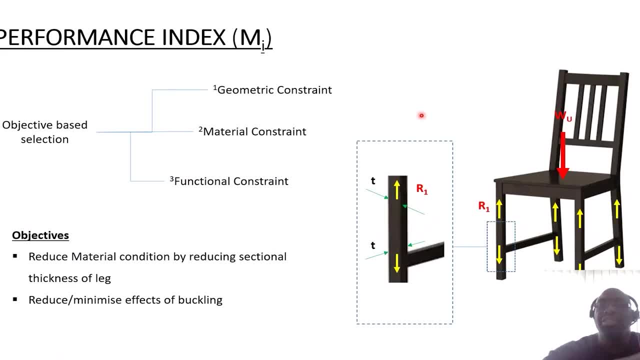 let's look at another example. so this brings us to the example that we looked at last week. so last week we used the constraint based model to identify the material and best for the design of the chair leg, assuming that there's going to be, you know, variation in the thickness. 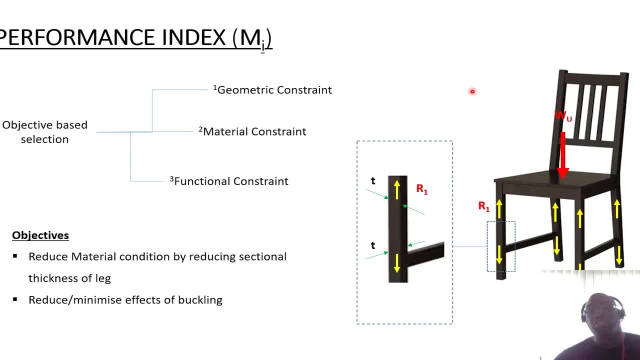 so from that particular tool we realized that the smaller the sectional thickness would be, the higher the value of a. but what is the caveat to that? the higher the stiffness, the more difficult it would be to fabricate. so we need to look at, you know, the material that gives the ideal balance in terms of 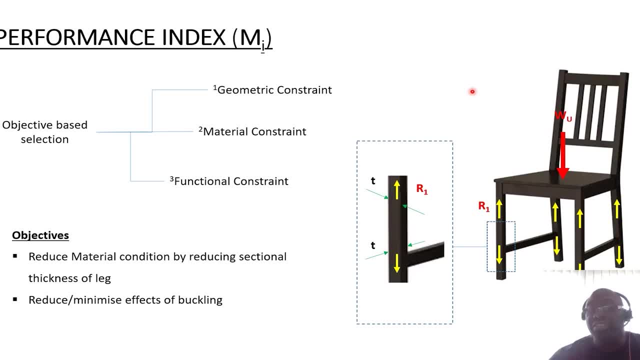 ideal uh resilience to buckling. ideal sectional thickness, so that you're not increasing the lading weight of the unladen weight of the chair. you also need to think about you know how light the material also needs to be. when it comes to this particular activity, we're going to look at using ces. so cs uses an objective based model where 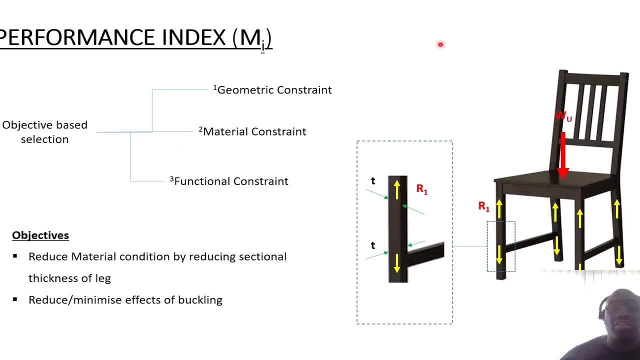 the material constraint tends to be the focus. so the constraint base. we focus on the functional constraints and the geometric constraint. but when it comes to objectives based modeling, the geometric and function constraints are fixed. so your variability will be via the material. so these are the objectives. so to reduce the material condition: 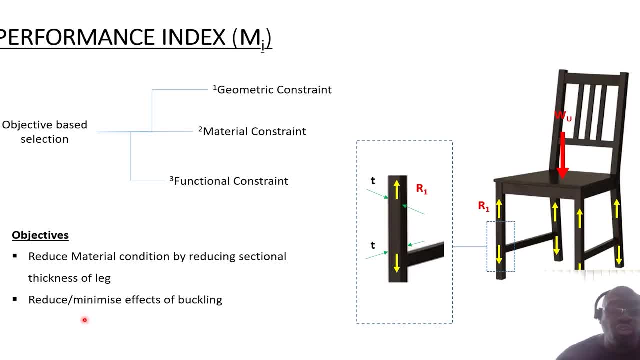 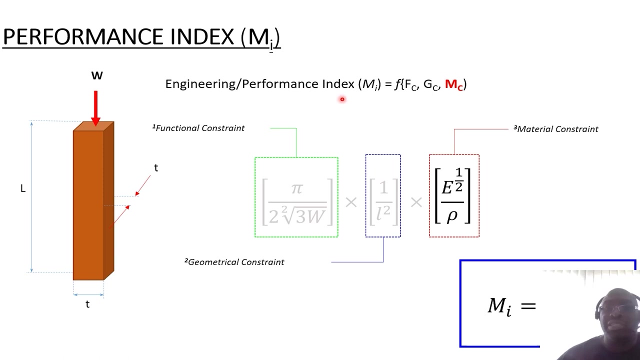 by reducing the sectional thickness of the leg, and to also minimize and reduce the effects of buckling. so we're trying to increase the material's resilience to compressive loading. so, as stated at the beginning, um, the engineering performance index, is the function of the functional, geometric and material constraint, but when it comes to cs, the emphasis is on the 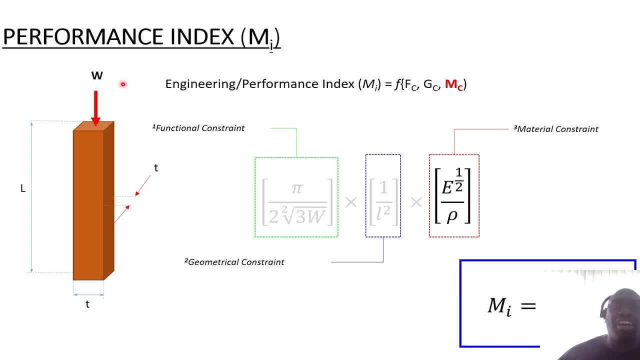 material constraint. so for us to analyze the effect of how stiff the material is against the its compressive load due to how slender- uh, the section of variance needs to be. we're going to be looking at this index. so i've proved this in the previous example, but i'm not going to use 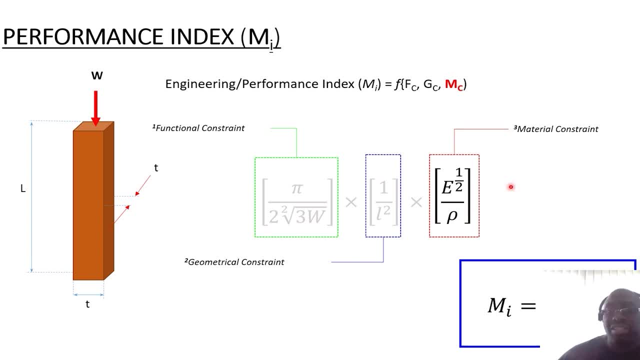 that because the mathematics is a bit complicated. but this is essentially the index and if you look at what's on cs, you realize that when it comes to looking at a similar model, this is the performance index that's been outlined. okay, so the performance index m will be equal to e, to the power half. 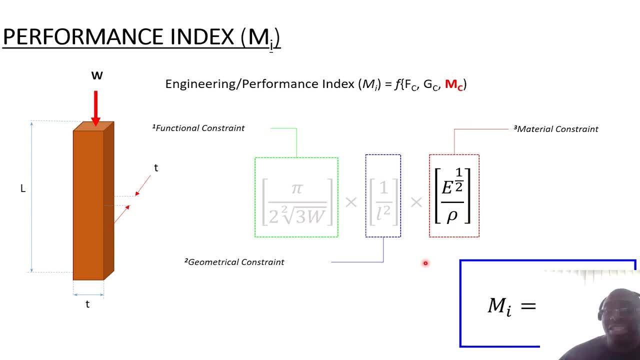 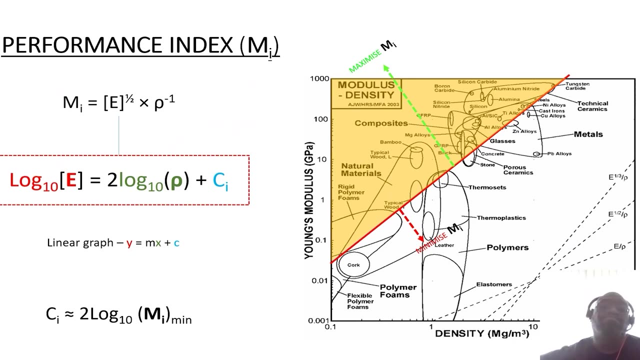 or the square root of e divided by the density. so we're going to look at a range of material that have similar characteristics, as defined by the performance index. so now that we've identified the best performance metrics to use, um, the whole idea is to now use that information to plot a graph. and once we've plotted the graph, 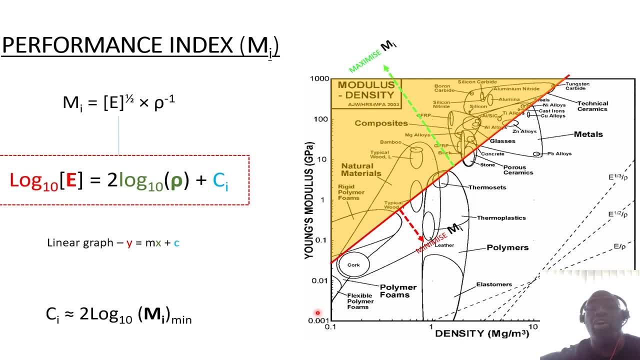 by means of identifying what would be the slope of the graph, we can then identify the range of materials, and that conforms to our design specification. so the whole concept when it comes to ces is, the further you move the graph leftwards and maximize it, if you move the graph rightwards, you're then minimizing m. so the whole objective is to 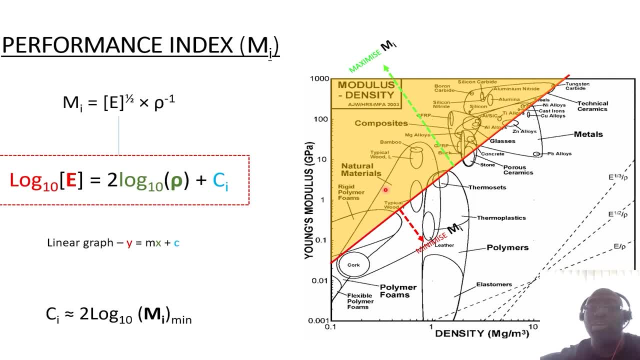 maximize m to give you the best performance that conforms to the performance index. so if you're looking at stiffness to density, if you move it leftwards the density that's characterized by the x-axis reduces. so again, the smaller the value of the density, the lighter it will be, and if you move in in that vector, the higher the young's modulus, the 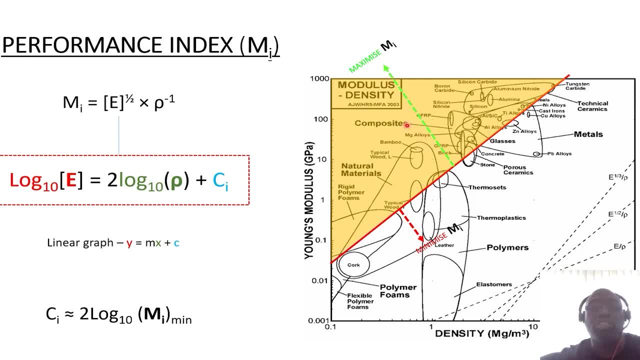 stiff of the material will be. as i stated, you don't want the material to be excessively stiff. the whole idea is based on transforming the performance index using logarithm to define the equation as a linear graph. so we know from first principles that you know the y-axis and the 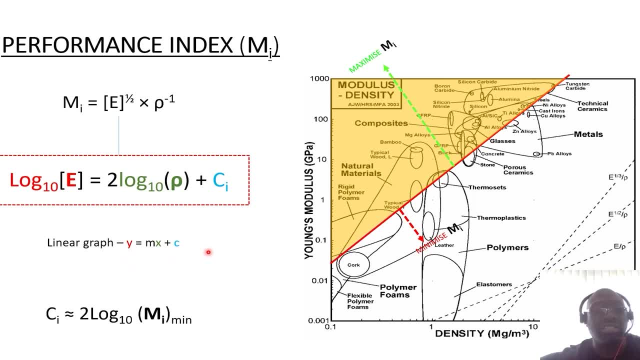 y-variables is dependent on a constant or the y-intercept, the gradient and the changes respect to x. when it comes to the slope, we're interested in the gradient. so, depending on what the performance in this is, it would define the nature of the slope. so back in my time, where we didn't 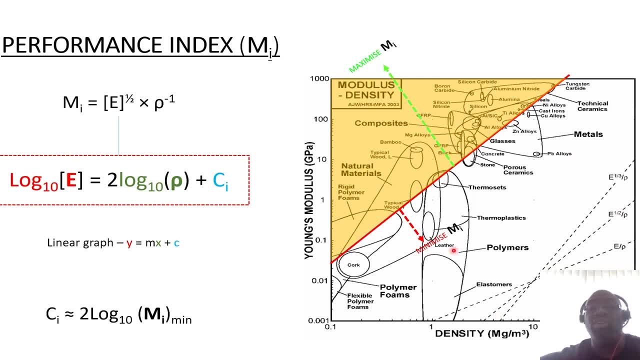 really have, you know, um the graphs converted into the software that you guys have at the moment. we had to use first principles to enable us, you know, plot any of the graphs- to identify the best material. um, moving forward, what i'm going to do is i'm going to compare, you know, the use of uh old 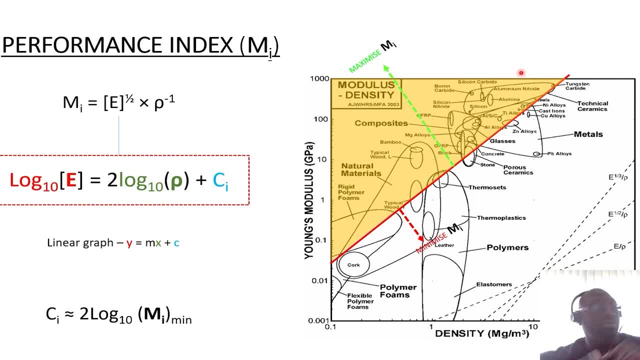 methodology and compare that to- you know, using the software, to see if we come to the same conclusion. so, based on what i have here is indicated that the range of materials that best conforms to um the design of the bicycle frame constitutes of rigid polymer foam. we've also got natural materials such as wood, whether it's high, soft bamboo. 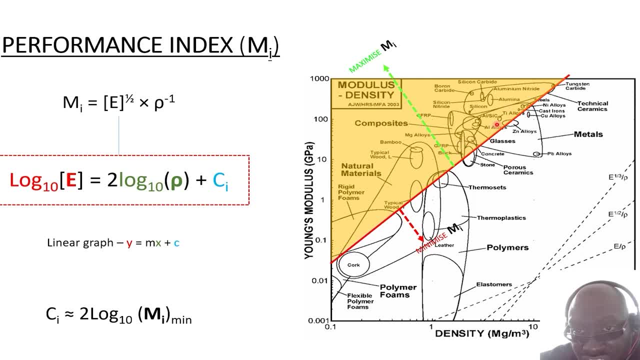 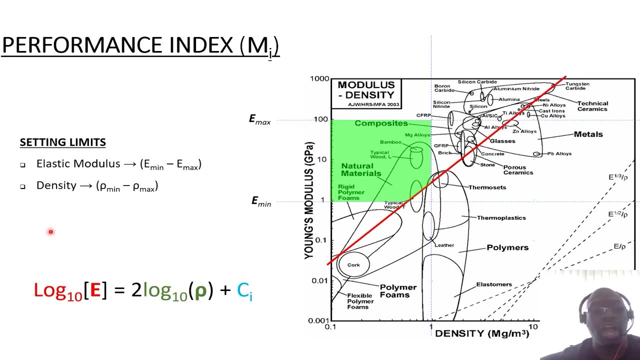 but we also got some technical ceramics and, technically, serrat are very difficult to machine, so we have to do a bit more to filter out our range. so this is where we apply what's called limits. so what i can do is i can create a limit in terms. 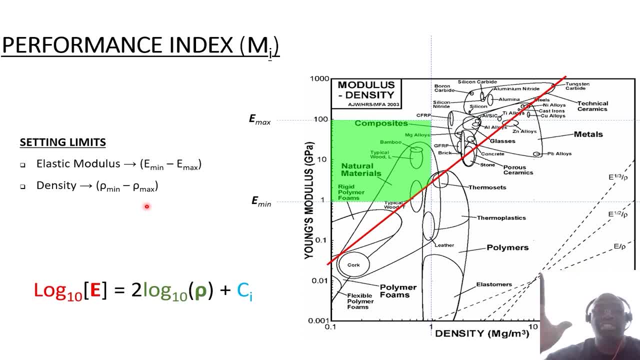 of the density. so what range of materials in terms of the density am i interested in? i can do likewise in terms of the elastic modulus. so what's the minimum stiffness i desire from the material? what is maximum stiffness that is designed in terms of the materials that we do select? so here, 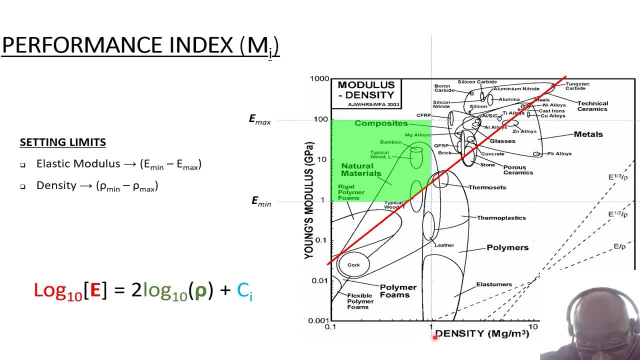 the limit i set for the density is looking at materials that have densities equal to a thousand kilograms per meter cube or less. okay, so based on that, i drift the graph, you know, leftwards to maximize what m will be, and i also set limits in terms of what the minimum desired elastic modulus needs to be. so this is set at one gpa and the 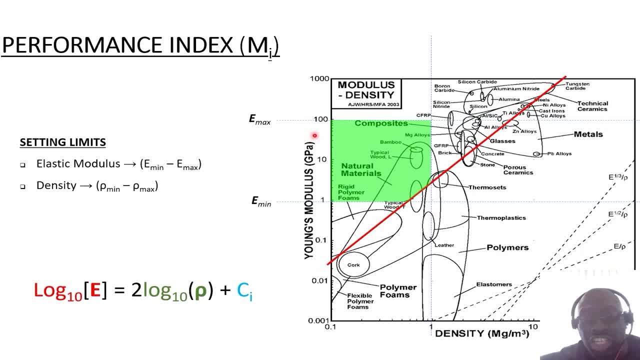 maximum um set just under a hundred uh gpa. so by introducing the limits, that then filters out uh the technical, uh ceramics, because that's a state to be quite difficult to machine and fabricate, thus making you know, processing and the ceramics very, very expensive. and it also eliminates uh the foams because particularly with the uh 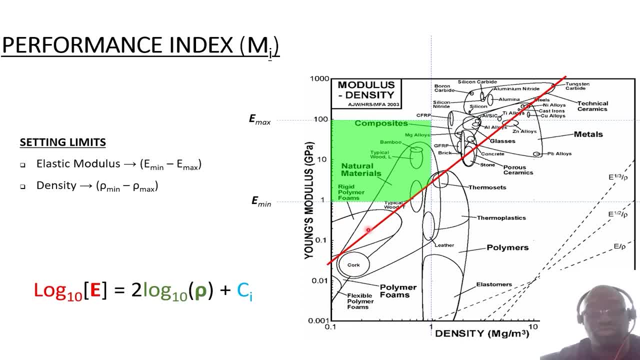 ceramic foam, still not very um strong and also, if it were to be metallic, very difficult to machine. so that's filtered out um everything and we're left with natural materials. so your bamboos, your woods, things like that, so okay, so this is basically what um is indicated, that's i inferred. 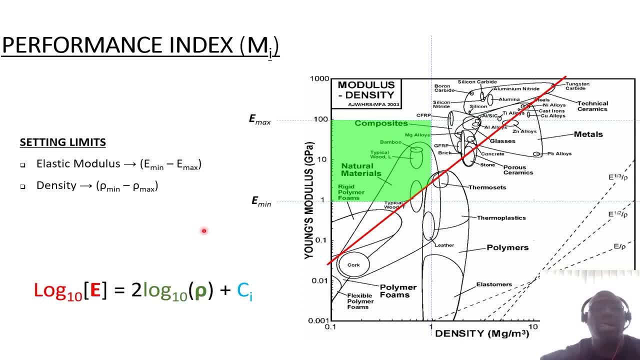 in the last tutorial. you can't limit um your decision on materials. so then you need to think about the operational parameters over time. you might need to think about the manufacturing uh implications. you need to expand that range because, again, you need to think about the operational parameters over time. 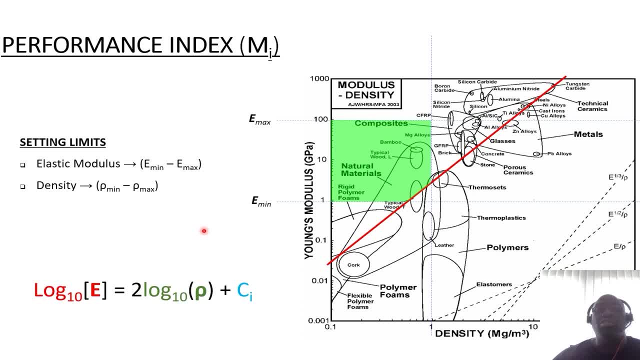 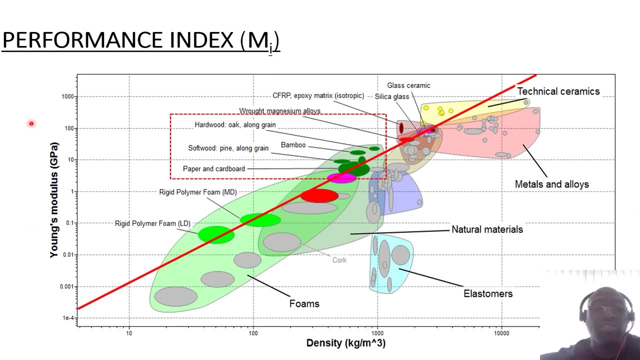 you might need to think about what the manufacturing implications are and other factors to enable you to make you know the right decision. uh, moving forward in terms of the best material that's suited for your product, selected software. So similar to the example I just shown, mapping the Young's. 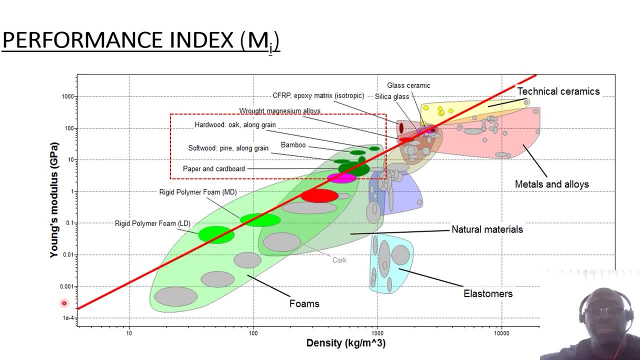 models that characterize the stiffness of the material to the density, and by identifying the slope of the graph to be 2, it then automatically introduces the line graph. So, by using the mouse, you can then drift the graph to wherever you want it to be. So, by drifting the graphs into the position and what I did using 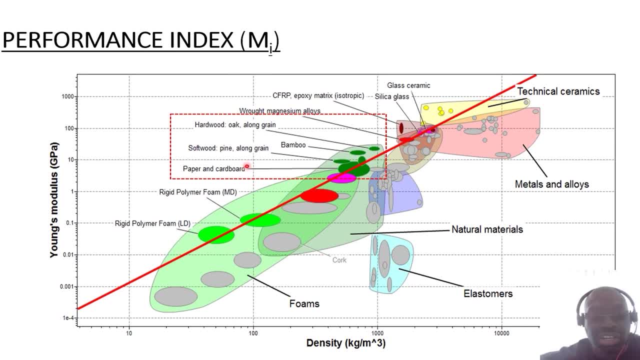 the old techniques, it's identifying similar material. So again, we've got our range of polymeric foam. we've also got our natural material selection that's constituted of wood, whether it's hard or soft, like oak, high and bamboo. It's also 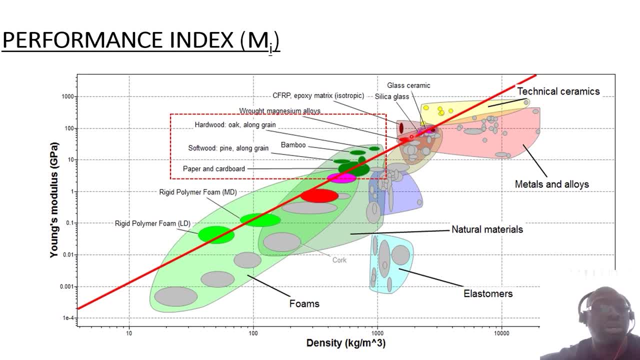 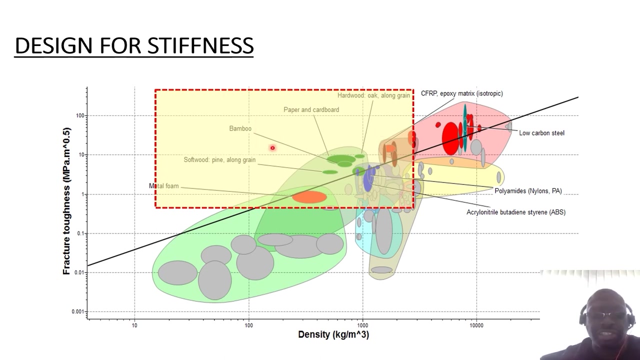 indicated some technical ceramics similar to the previous example. So what do we do? We then have to now introduce limits. So the more limits you use, the narrower the material field becomes. At the moment, our data and our metrics is indicated that bamboo is probably the best material to select. But, as I've inferred, you can't just base the 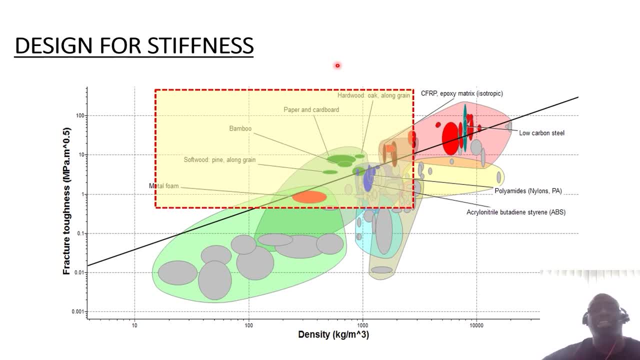 on the few criteria. you need to look at your design specification, to look at a whole range of criteria to enable you identify the best material of choice, because sometimes, if your focus is on you know the function of parameter- that's not necessarily me that it checks the. 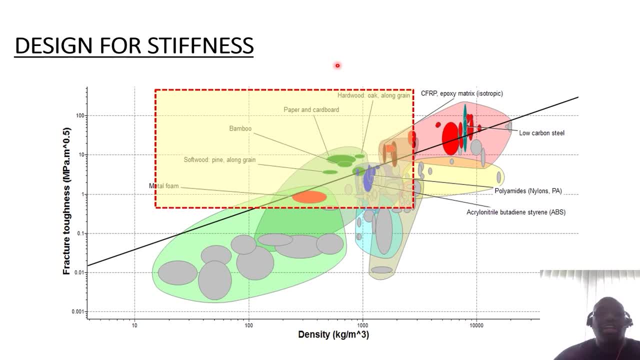 boxes when it comes to, you know, uh recycling or material recovery, and you know the needed manufacturing processes to you know yield um, the component that you're trying to design. so you may have to look at other parameters too to enable me confirm whether bamboo is the ideal choice for. 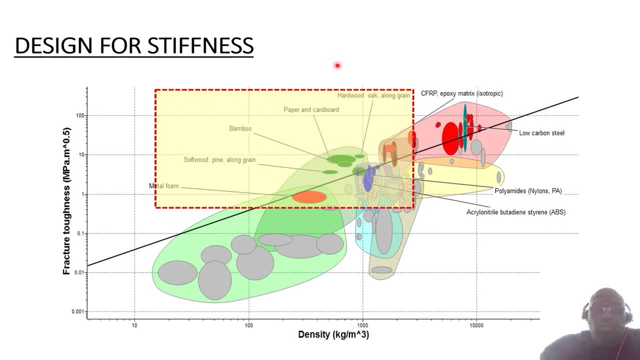 the bicycle frame. i'm going to now look at another property called fracture toughness. fracture toughness is basically a material's capability of, you know, controlling or reducing the rate of crack propagation within its structure, as hopefully you guys do know when you did your material module in year one. when it comes to the transformational material from its prior, from its raw state to its